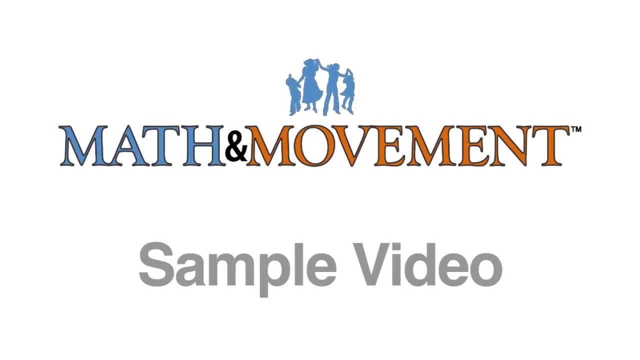 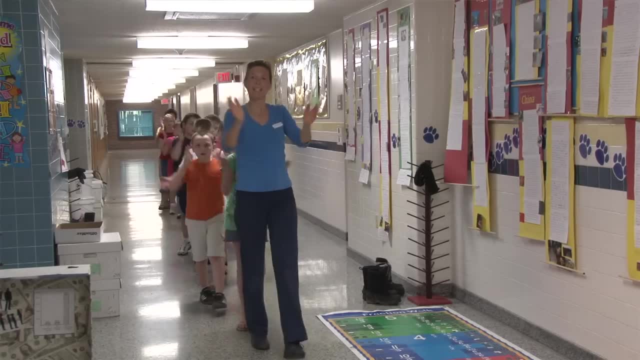 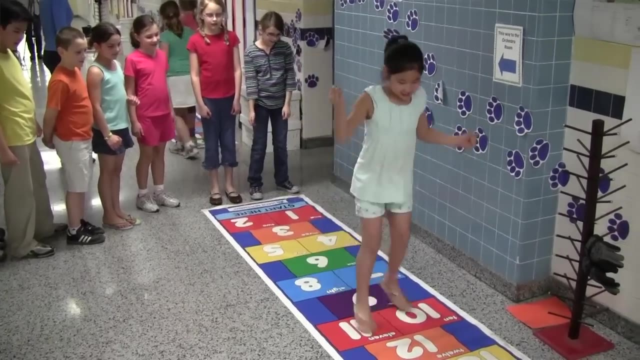 I like math and movement because it's a way to get really active and physical shape, while you also get to learn a lot of math, and it's just a fun way to learn math and express yourself. This is jump box fours. The first thing to do is to jump with your right foot forward. 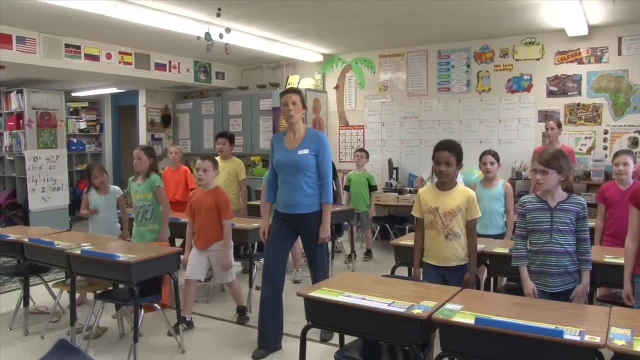 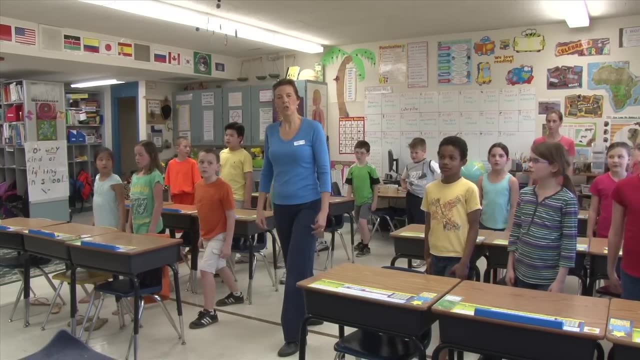 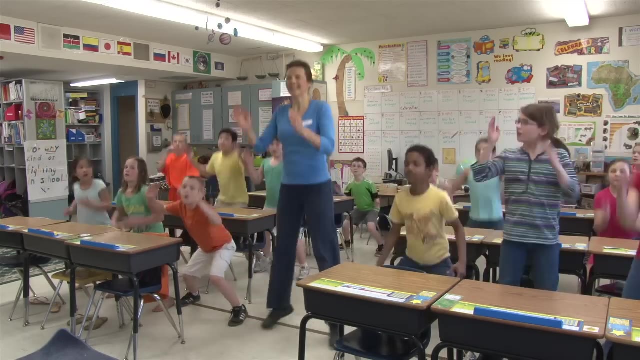 and your left foot back and whisper one And then switch legs and whisper two, Then jump with a straddle and whisper three And jump together and clap four. I think math and movement is a really good skill for kids that think math is like really. 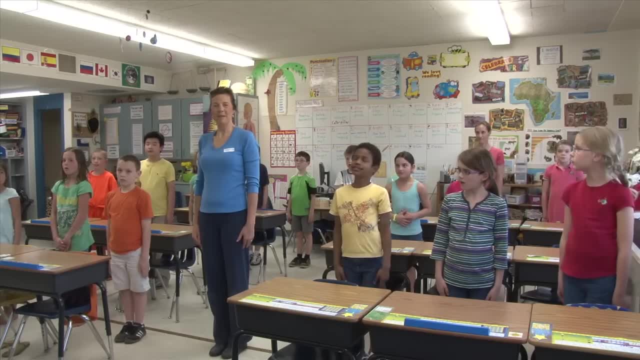 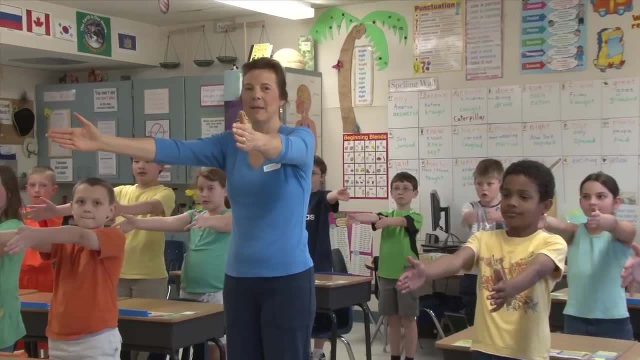 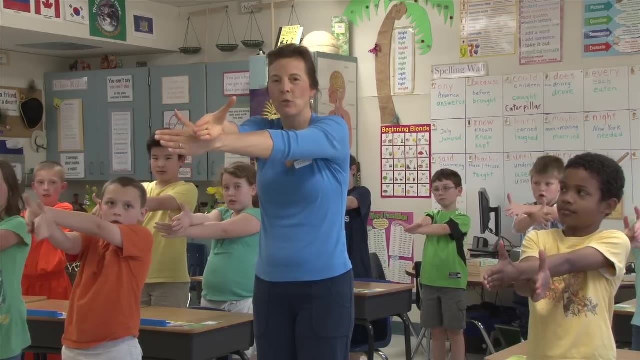 boring. Math is funner than you think. This is elephant march. The first thing that you do is to put your hands straight out, clap them together, cross one over the other. Now take your thumbs and turn them up and now turn them down, Interlock your fingers and 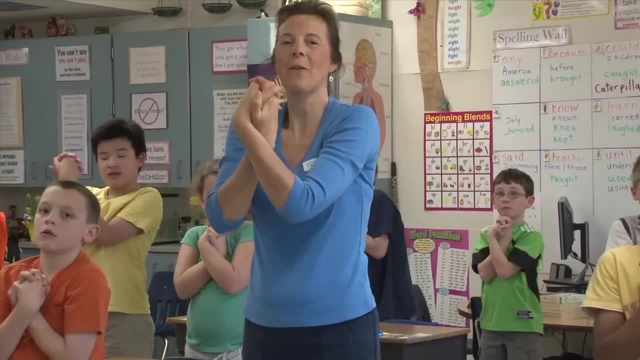 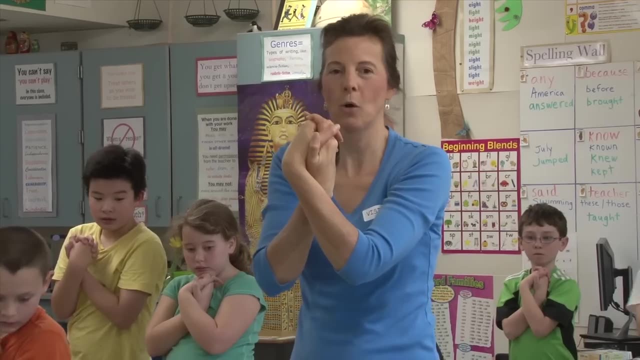 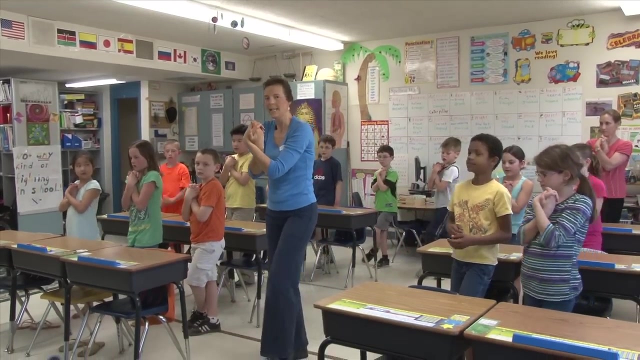 scoop like an ice cream cone. This is our elephant's trunk and we're going to do the elephant march. The first thing to do is to take your right foot and cross it over your left and whisper three. One. Then your left foot and over your right and whisper two, Then raise your elephant's. 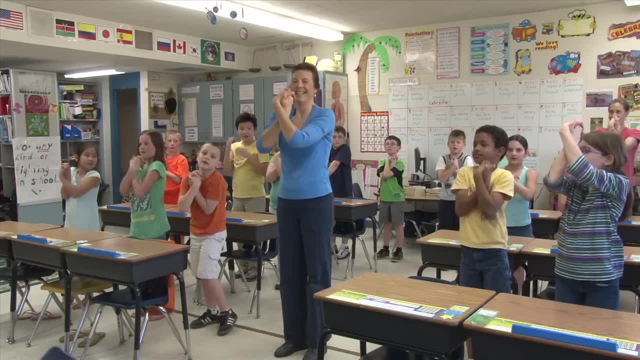 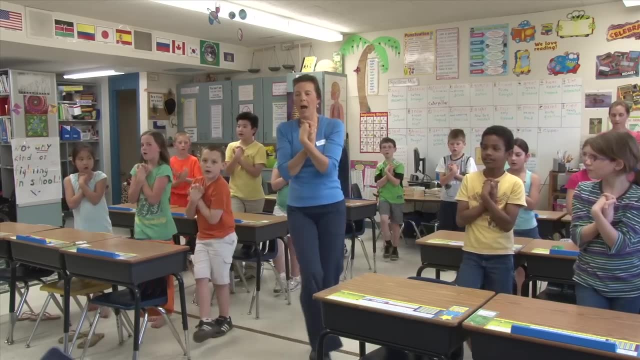 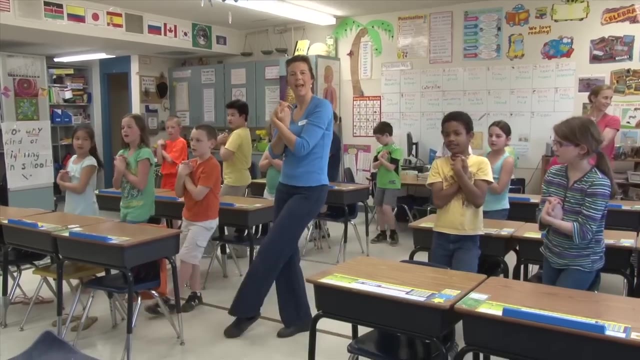 trunk and say: three, You got it, Let's go Ready set go. One, two, three, four, five, six, seven, eight, nine, ten, eleven, twelve. three, four, five, six, seven, eight, nine. 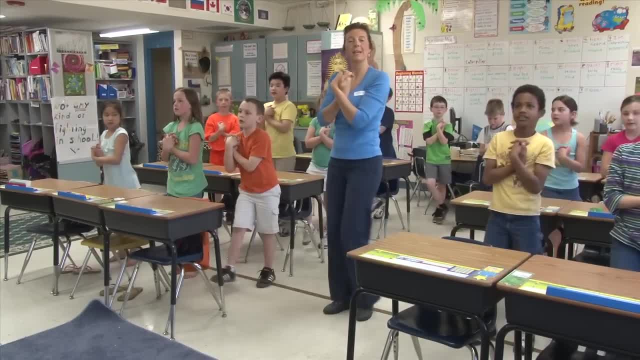 ten, eleven, twelve, three, four, five, six, seven, eight, nine, ten, eleven, twelve, thirteen, fifteen, sixteen, seventeen, eighteen, twenty-one, twenty-two, twenty-four, twenty-seven, twenty-eight, twenty-nine, thirty. 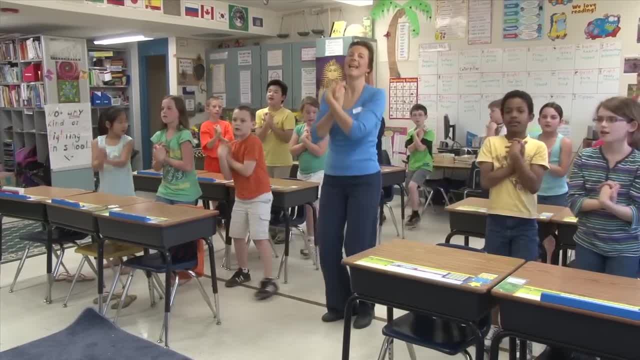 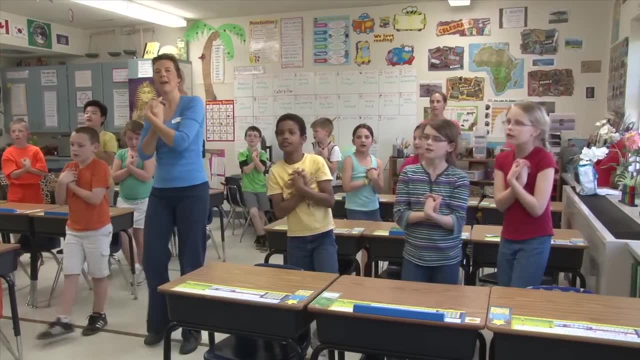 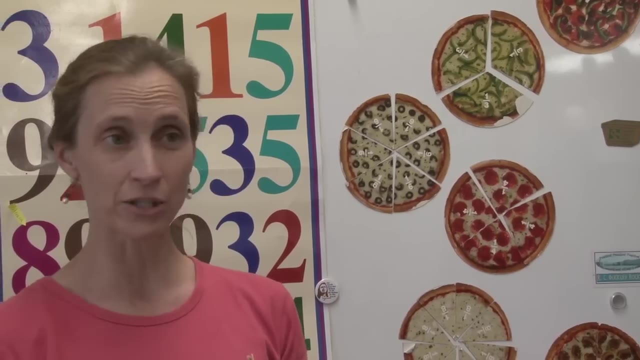 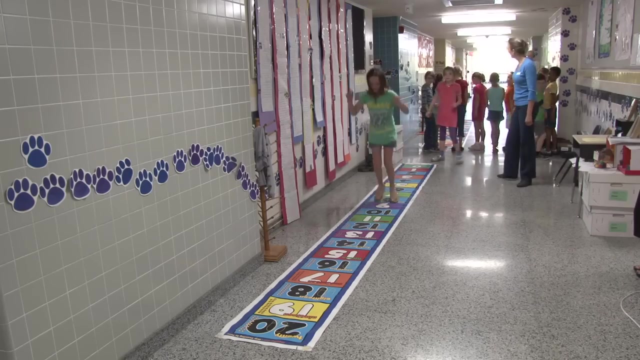 I mean normally when kids count, they do it by rope and don't think about it, But somehow when they're moving their body to the left and the right at the same time, it really involves the brain. It's a good workout and it's fun.